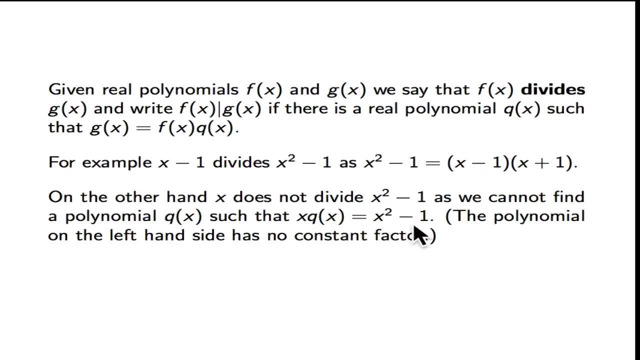 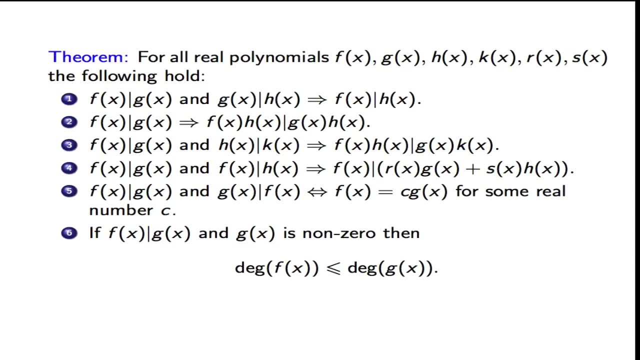 such that x times q is equal to x squared minus 1.. For example, the polynomial on the left-hand side has no constant factor. The polynomial on the right-hand side has constant factor equal to minus 1.. And the next theorem is analogous to the theorem we had for the divisibility. 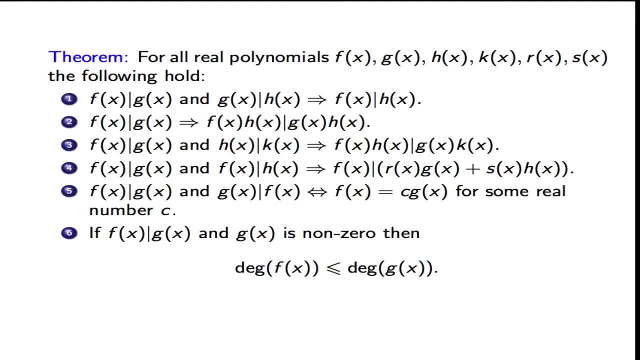 of integers. So this one says that if we have real polynomials f, g, h, k, r and s, then the following works: If f divides g and g divides h, then f divides h. If f divides g. 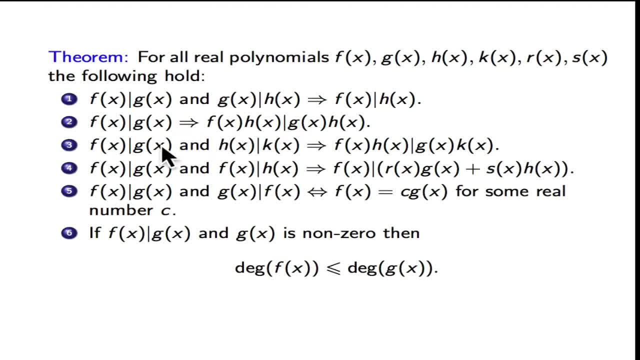 then f times h divides g times h. If f divides g and h divides k, then f times h divides g times k. If f divides both g and h, then it divides any linear combination of g and h, And by linear combination we mean: 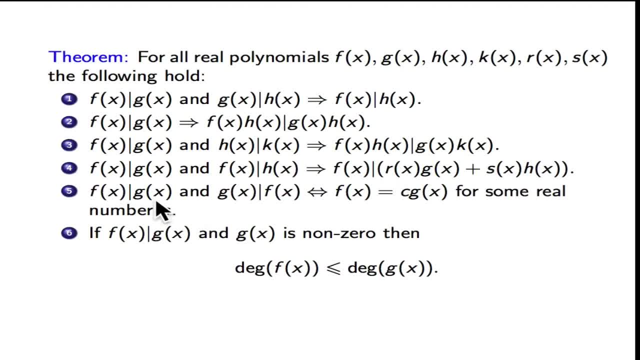 polynomial linear combination. If f divides g and g divides f, then f of x must be equal to constant times g of x for some real number, c. And if f of x divides g of x and g is not 0, then the degree of f is less or equal to the degree of g. 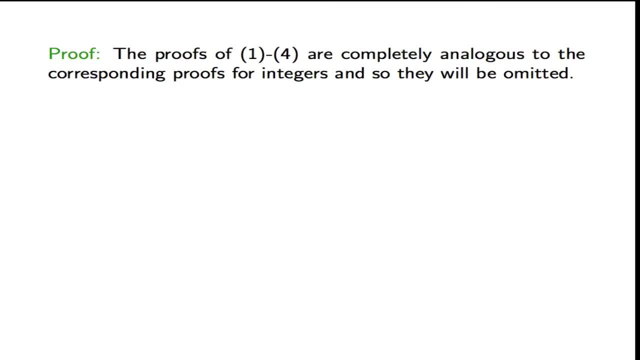 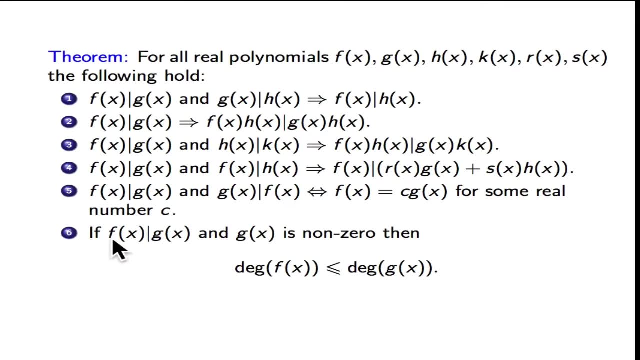 The proofs of one to four are completely analogous to the corresponding proofs or integers, So we will omit them And we'll only prove 5 and 6.. So remember, 5 says that if f divides g and g divides f, then f must be equal to c times g. 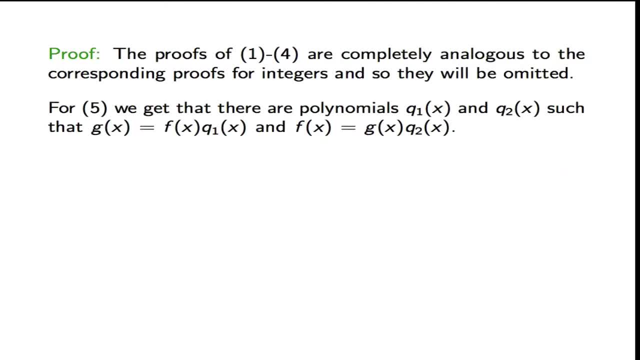 for some real number c. But if f divides g and g divides f, then we can get polynomials q1 and q2, such that g is equal to f times q1 and f is equal to g times q2.. And so g must be equal to g times q1 times q2.. 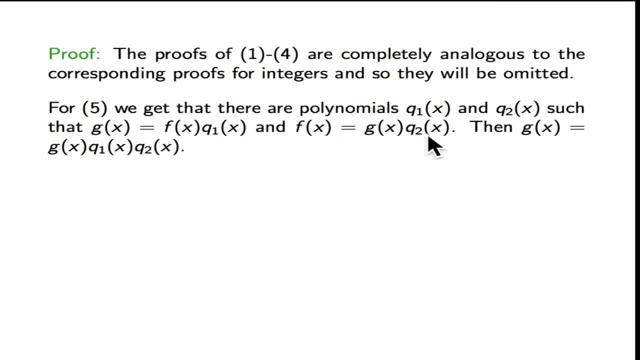 So we replaced f in this equation with g times q2.. And this gives that the degree of g must be equal to the degree of g plus the degree of q1 plus the degree of q2.. And this was from the theorem. we were saying that the degree of the sum of two polynomials 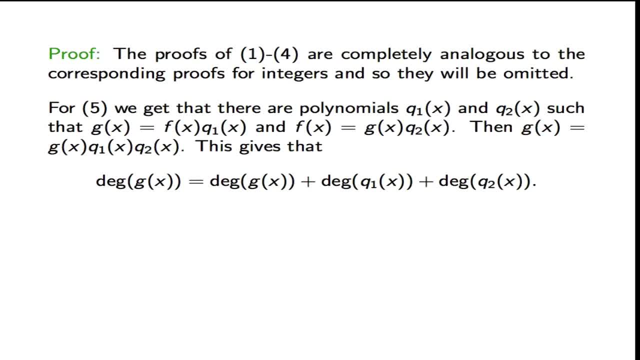 is equal to the sum of their degrees iterated for three polynomials. But then either g of x is a zero polynomial and we have minus infinity appearing as degrees, or if g is not the zero polynomial, then q1 of x and q2 of x must have degrees zero and 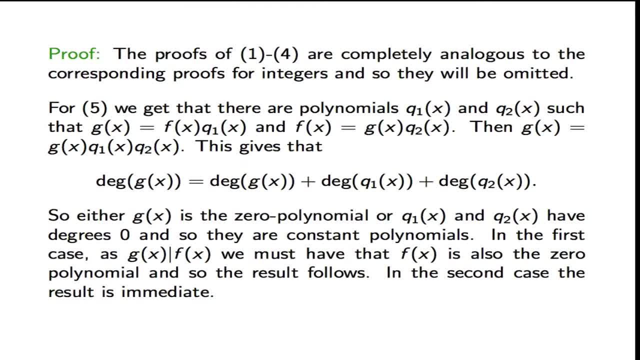 so they must be constant polynomials. Now, in the first case that g of x is a zero polynomial. so if g divides f, then we must have that f is also a zero polynomial And then the result follows, Because the result we wanted to show that f is equal to constant times g, and we did. 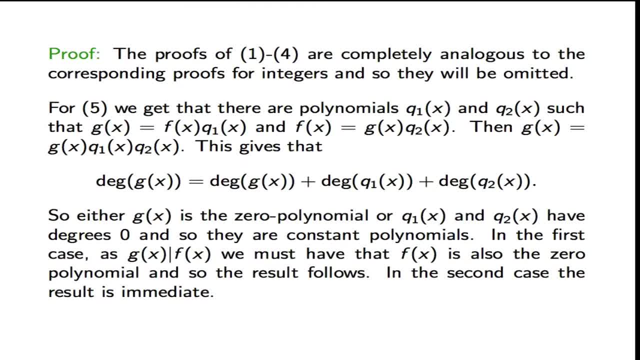 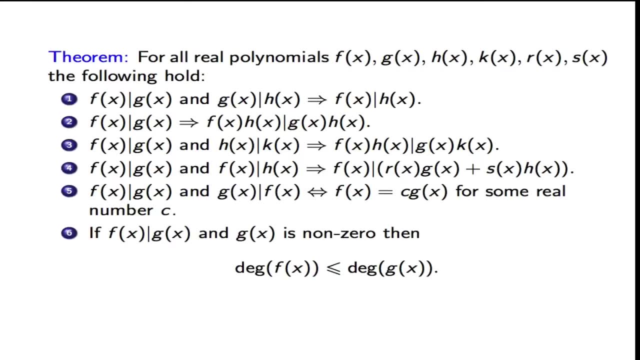 Because both are equal to a zero polynomial, And in the second case the result is also immediate. We know that f is equal to q2 times g, but we have shown that q2 is constant. Okay, so let us now move to 6.. 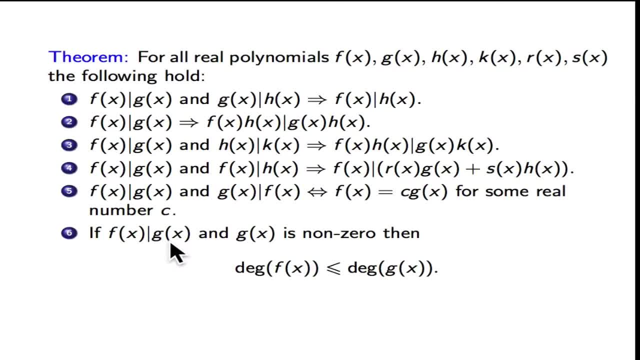 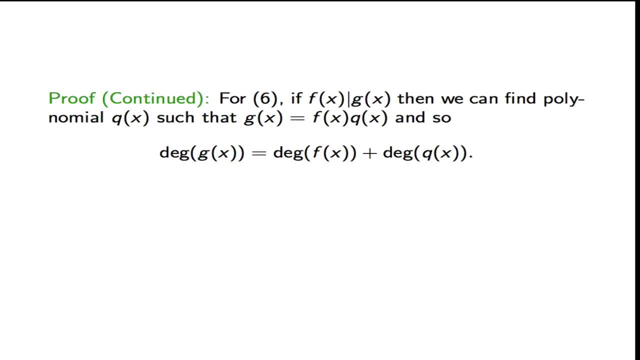 Let's remember. it says that if f divides g and g is non zero, then the degree of f is less than or equal to the degree of g. Okay, we know that f divides g, so we can find a polynomial q such that g is equal. 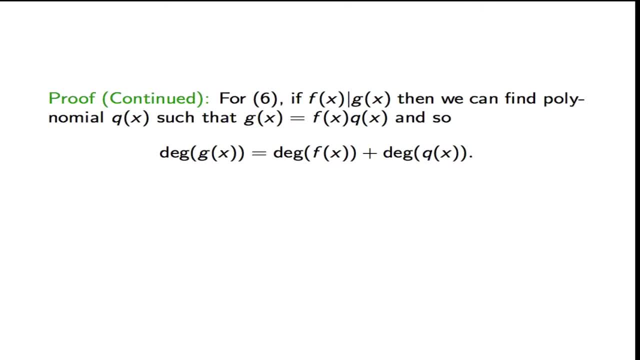 to f times q, And so, since the degree of the product of two polynomials is equal to the sum of their degrees, then the degree of g is equal to the degree of f plus the degree of q, And therefore the degree of g is indeed greater or equal to the degree of f, as required. 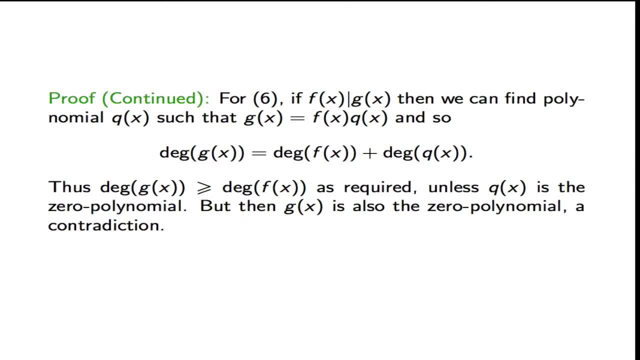 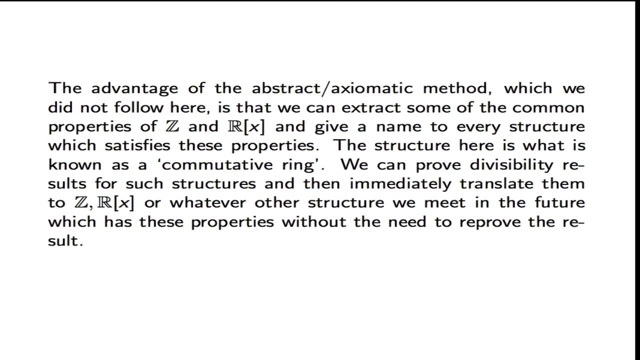 unless it so happens that Q is a zero polynomial. This is an extra case that we need to consider. But then if Q is a zero polynomial, G is also the zero polynomial which we have already excluded. at the beginning We said that G was a non-zero polynomial. Now the advantage of the abstract and axiomatic. 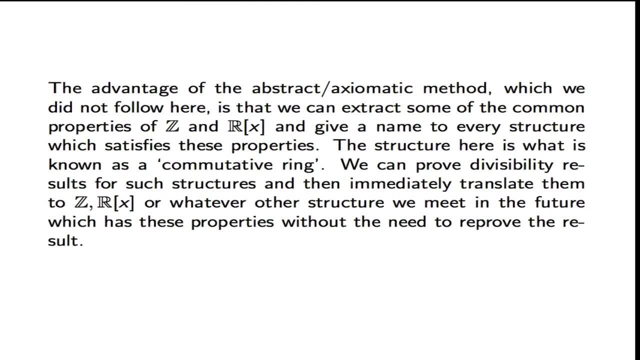 method which we did not actually follow here is the following: We can actually extract the common properties of the integers and the real polynomials and give a name to every structure which satisfies these properties, And actually the name we give to such structure is a cumulative ring. So a cumulative ring is: 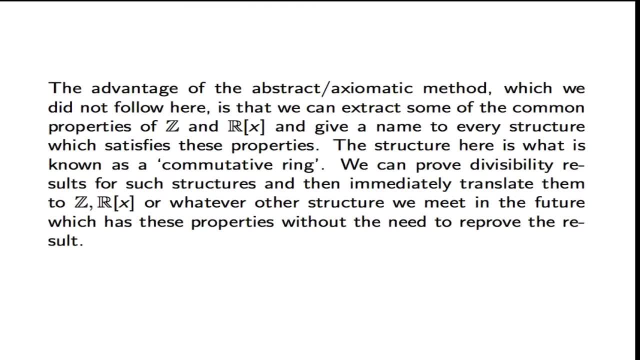 something that satisfies some properties, and those properties are actually some common properties of the integers and the real polynomials. Then what we can do is we can prove divisibility results for such structures And this we can immediately translate them to the integers, to the real polynomials, or 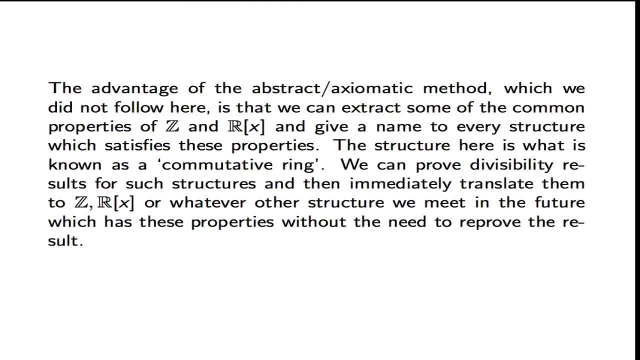 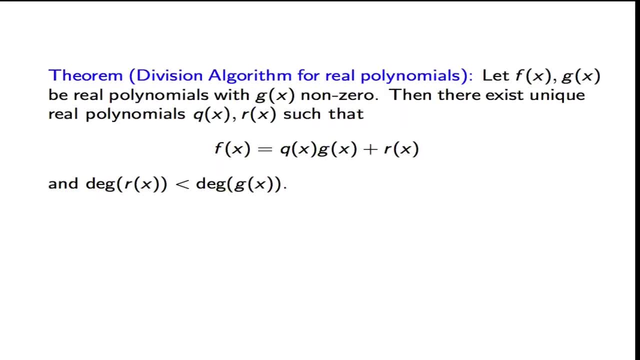 whatever abstract structure we ever meet in the future which has these properties, And we don't actually need to prove these results again. Okay, so let's proceed now with the division algorithm for real polynomials. Suppose we have two polynomials, f and G, with G being non-zero, And the claim is that there 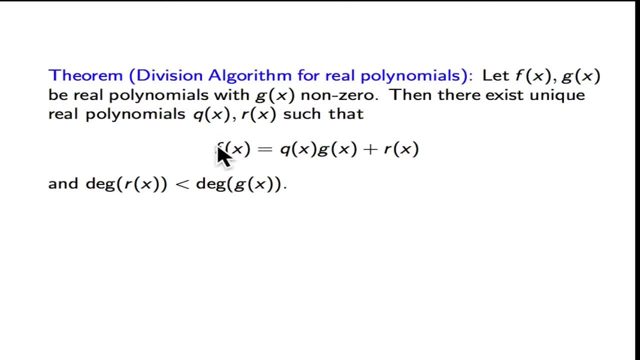 exists unique real polynomials, Q and R, such that f is equal to Q to the times G plus R, with the extra condition that the degree of R is strictly less than the degree of G. And naturally we call Q the quotient and R the 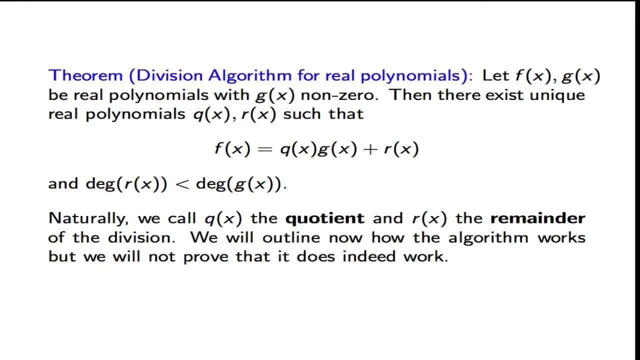 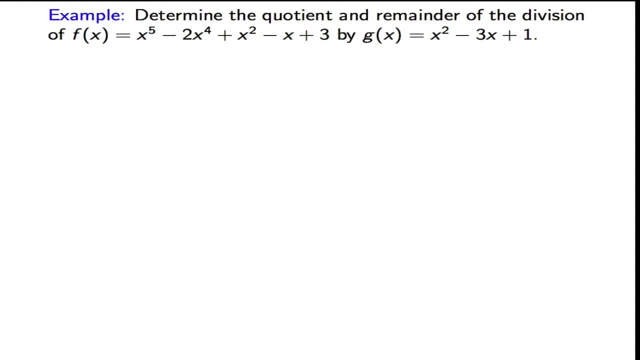 remainder of this division. We will now outline how the algorithm works, but we will not actually prove that it does indeed work. Okay, let's see an example. Suppose we want to determine the quotient and the remainder of the division of f we. 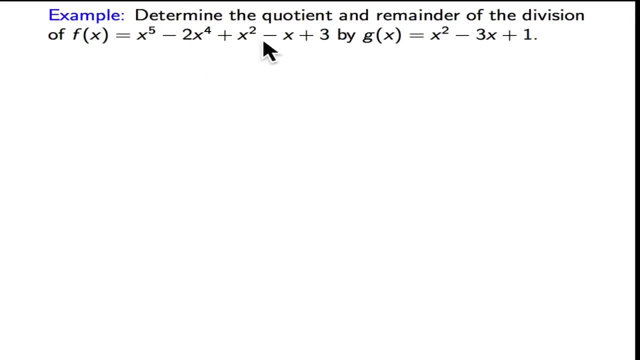 choose equal to x to the 5 minus 2x, to the 4 plus x, square minus x plus 3, find G, which is equal to x square minus 3x plus 1.. So the first thing we do, we write f here, we draw a straight line up of it and we write G to. 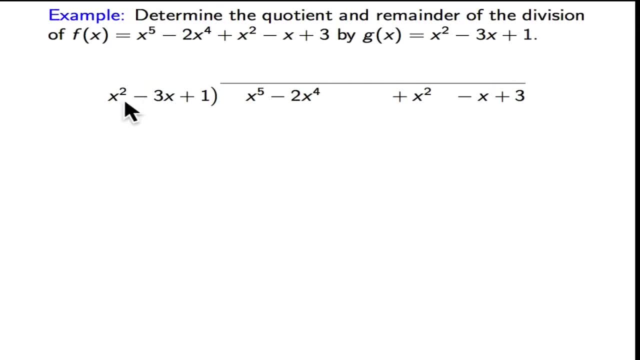 the left of it. The first thing we look is how many times x square goes into x to the 5. And it goes exactly x cubed times. So we write x cubed here. Note that we have left some space when we've written f. 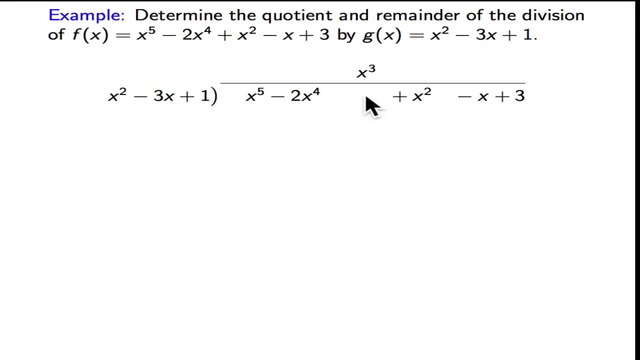 of x, because the degree, the coefficient of x cubed was zero. So don't write x squared right next to 2x to the 4 minus 2x to the 4, because then you will have problems. Okay, so x squared goes x cubed times into x to the 5.. The next step is: 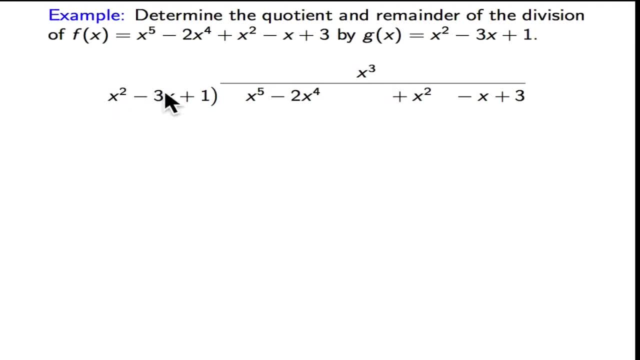 to do the multiplication of x cubed with x squared minus 2x to the 5.. So we have written x squared minus 2x to the 4 minus 3x plus 1. And write it here. but instead of writing the multiplication of x cubed with this, we write the negative result. So 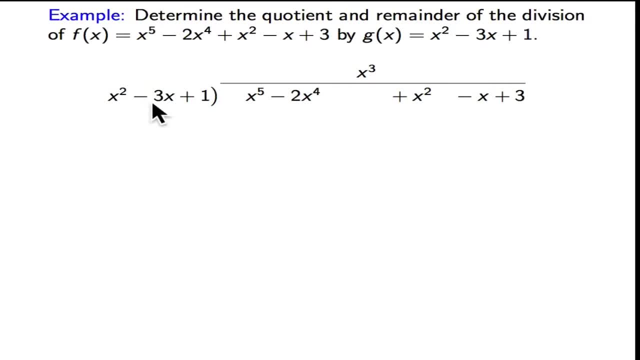 essentially we write the multiplication of minus x cubed with x squared minus 3x plus 1.. So we've written down: so x cubed minus x squared is x to the 5.. We've written minus x to the 5. x cubed times minus 3x is minus 3x to the 4. We've written plus 3x. 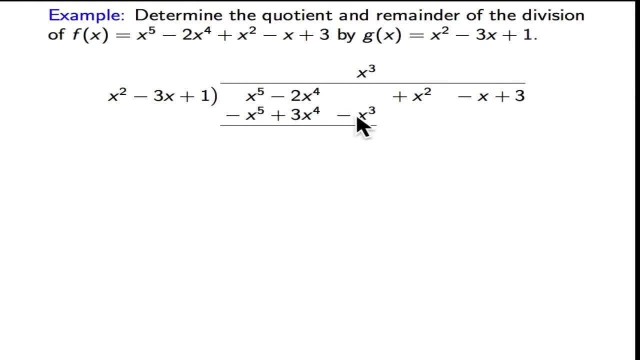 to the 4. x cubed times 1 is x cubed. We've written minus x cubed And now we add this polynomial with this polynomial And notice that the important thing is that the x to the 5 terms cancel now because we have 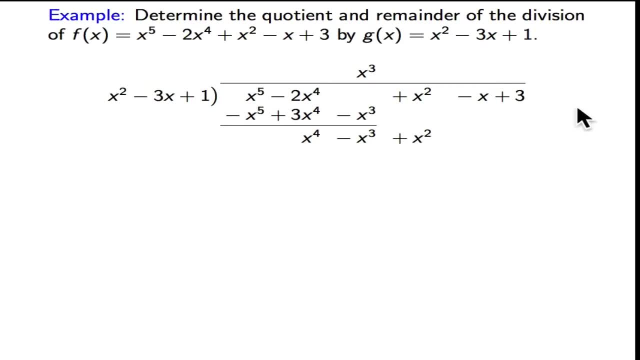 an x to the 5 and a minus x to the 5.. And actually it's not necessary to bring down everything. It's enough to bring down now only the next term, the x squared term. Okay, Now we look how many times x squared goes into x to the 4. x squared times. So we have 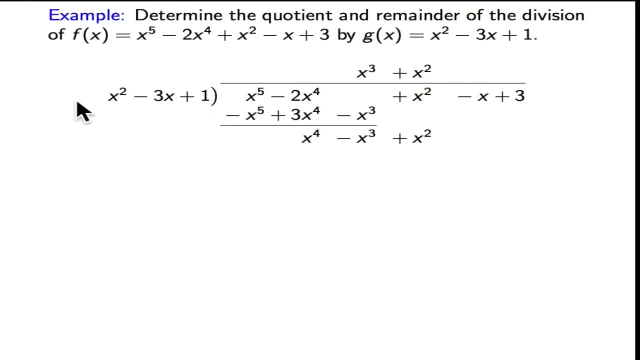 x squared times. So now we multiply x squared with x squared minus 3x plus 1. Write the negative result here, Add the 2. Bring the minus x down. Now look how many times x squared goes into 2x, cubed 2x times. Multiply 2x with x squared minus 3x plus 1. Write the negative, Add. 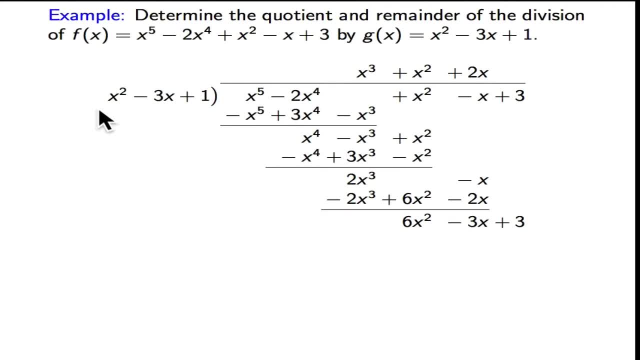 Bring the 3 down. Check how many times x squared goes into 6x squared. 6 times Multiply 6 with x squared minus 3x plus 1.. Write the negative, Add, And now this is the final step, and the quotient turns out to be this number, here, This polynomial. 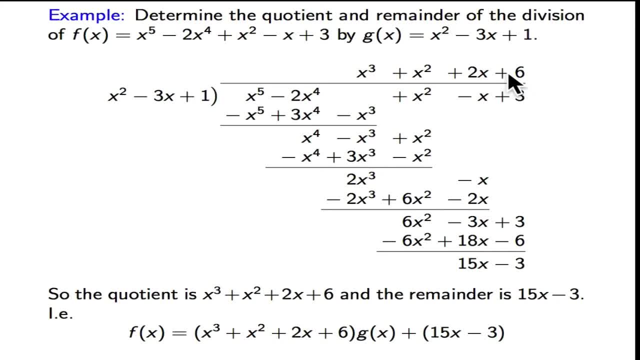 here x cubed plus x squared plus 2x plus 6.. And the remainder turns out to be the 15x minus 3, which has indeed its degree, is indeed less than the degree of g, And so we can actually write f of x being equal to x cubed plus x squared plus 2x plus 6 times u of x plus 15x. 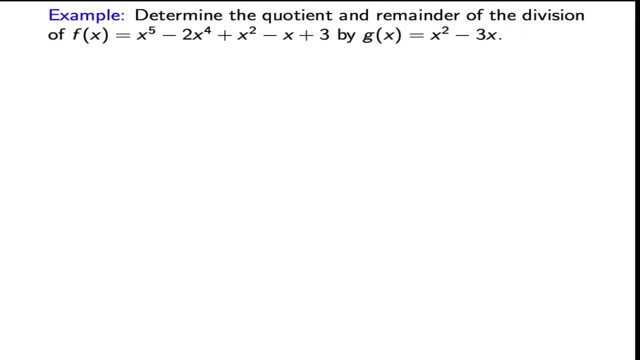 minus 3.. Let's see another example. Again, we want to determine the quotient and remainder of the division of two polynomials. Again, we write f here, g here and we start by looking how many times x squared goes into x to the 5th And it's x cubed times. we multiply x. 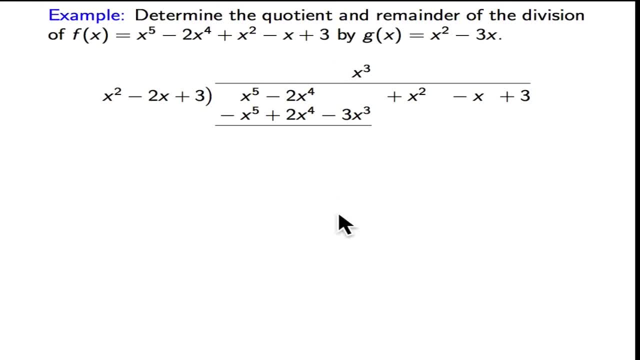 cubed by the polynomial. we write the negative of it, we add and now observe that the x to the 5th cancels, but also- it just happened- that the x to the 4th also cancels. So whenever this is the case, instead of bringing down only x squared, we bring another one term.